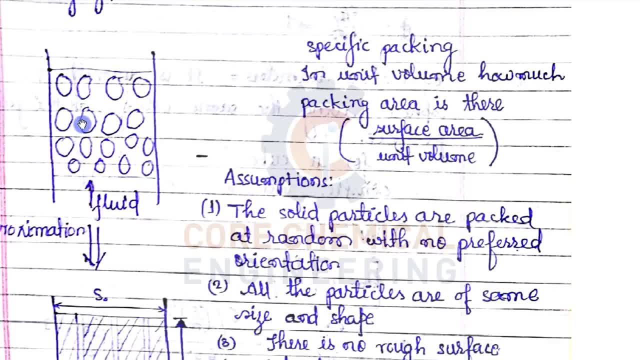 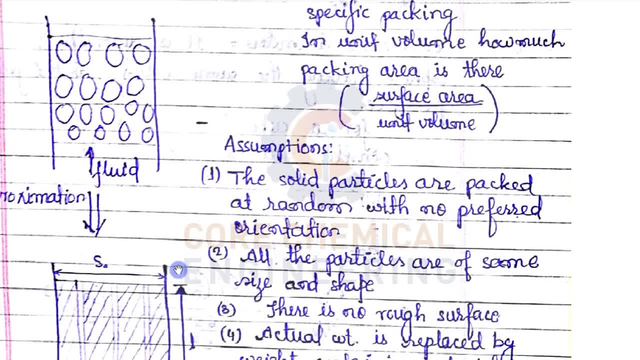 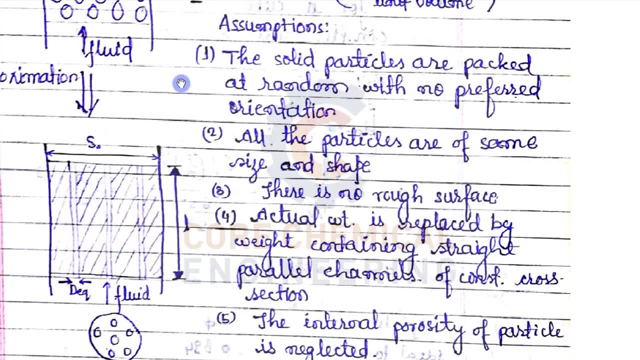 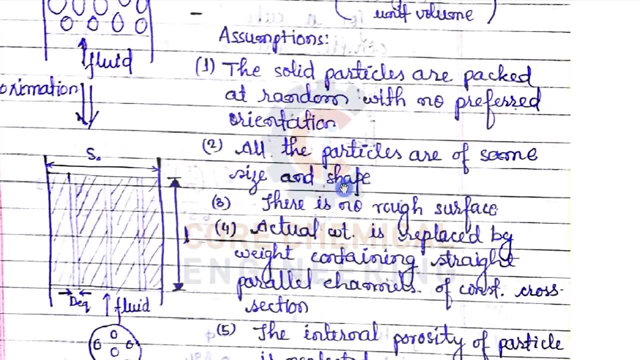 So, as we know, pressure drop through a bed of solid. So if we do the pressure drop, we are considering the following assumptions: the solid particles are packed at a random, with no preferred orientation. Now, all the particles are of same size and shape, But we are taking it as an assumption. 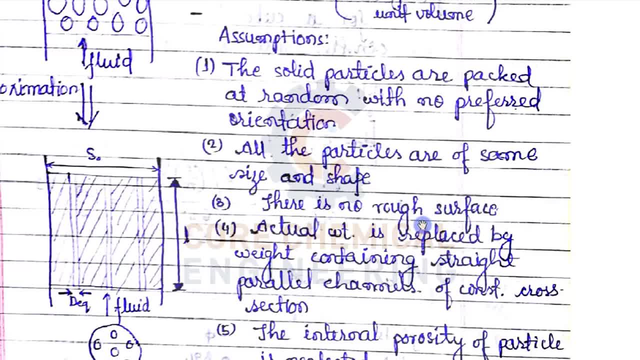 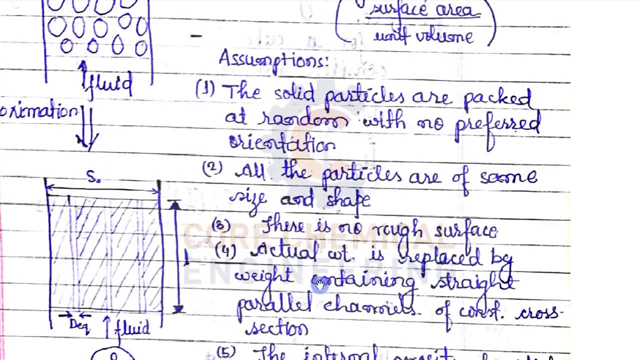 There is no rough surface. Obviously there will be rough surface. rough surface- we cant get 100% smooth surface, ok. fourth, actual bed is replaced by the bed containing straight parallel channels of constant cross section. so the actual bed, you can see it- is replaced by bed containing straight parallel channels like this: this is straight. 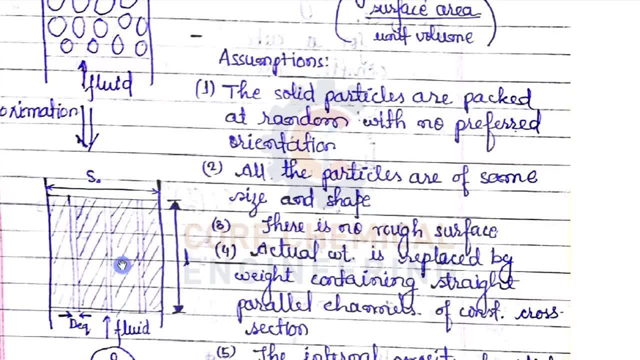 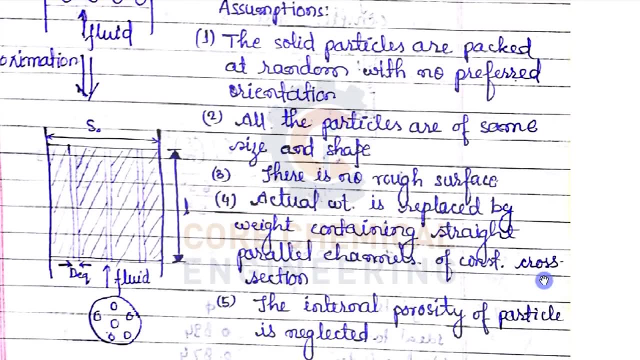 parallel channels. so this is the empty space through which now fluid will flow. ok, and these beds are actual bed are being replaced by these channels: 1, 2, 3, 4. ok, actual bed is replaced by bed containing straight parallel channels of constant cross section. now the fifth assumption. 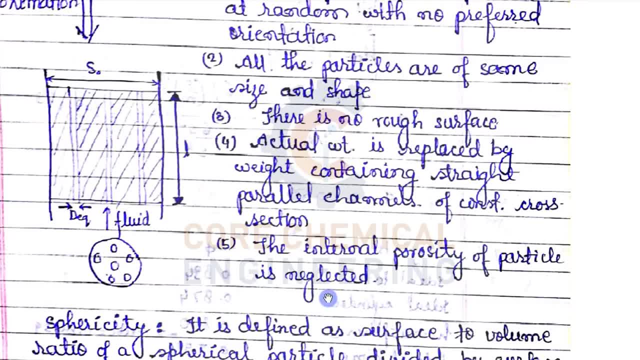 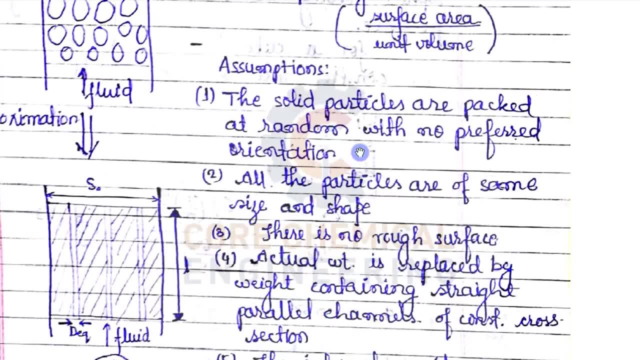 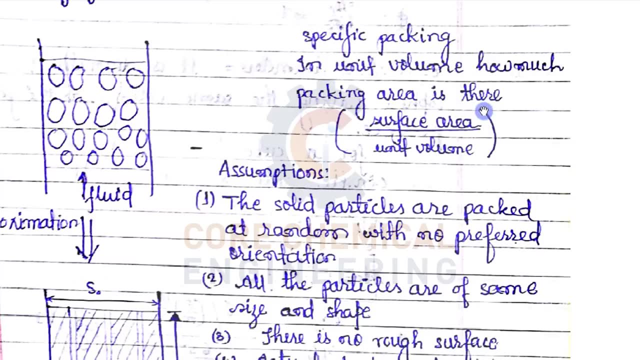 is, the internal porosity of particle is neglected, so internal, the particles which are arranged in this packed bed, the internal porosity of the particles are neglected. ok, now we will see one more thing. what is specific packing here? so, in unit volume, how much packing area is there is called specific packing, surface area. 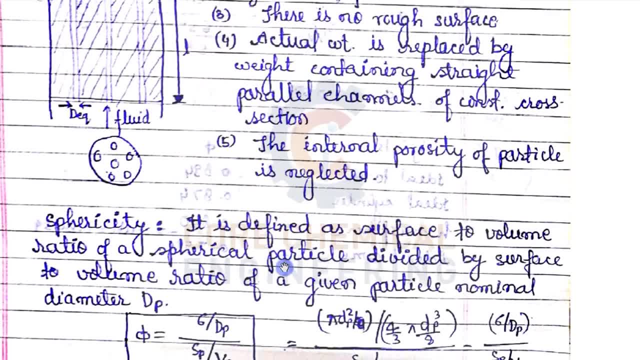 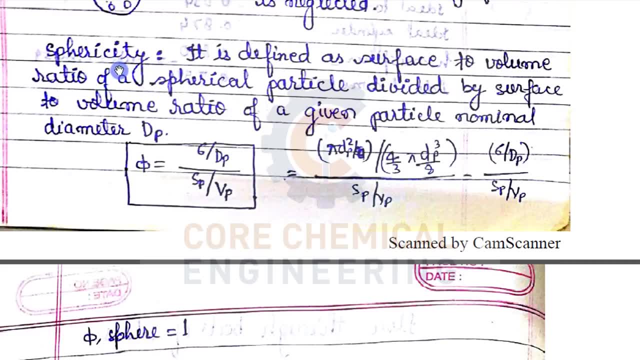 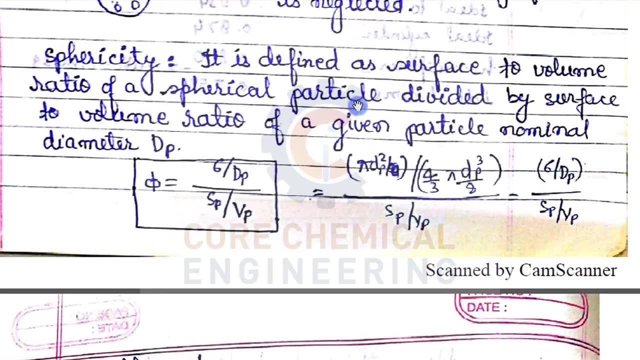 divided by unit volume. ok, now we will go for the derivation part. so before that, we need to know about sphericity. ok, and this is very important with respect to the gate exam. so sphericity is defined as surface to volume ratio of spherical particle divided by surface. 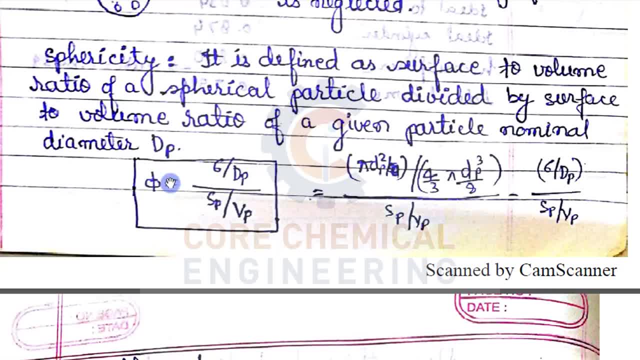 to volume ratio of a given particle: nominal diameter: 2. dp- ok, so the formula is equal to 5, is equal to 6 by dp divided by sp, by p, sp by bp. ok, sp is your surface area of particle, bp is the volume of the particle. here, 6 by dp. dp is: 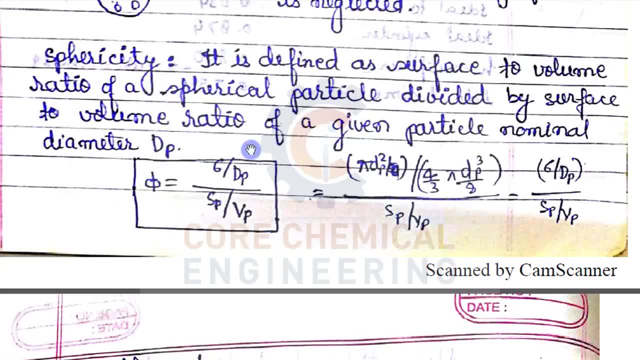 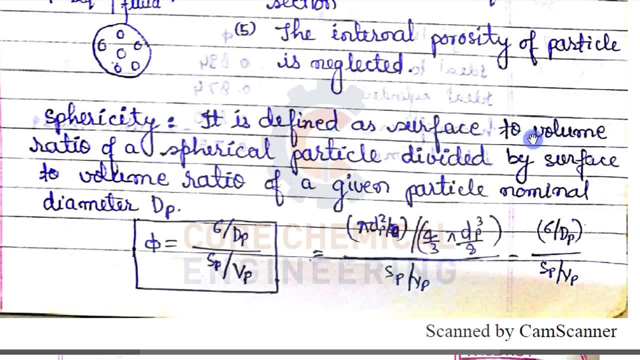 the diameter of the particle. so you can see that this derivation, this value, you can get it from here. ok, from the definition. you can see it here. it is defined as the surface to volume ratio of a spherical particle. the surface area, as you know, would be your pi dp square. 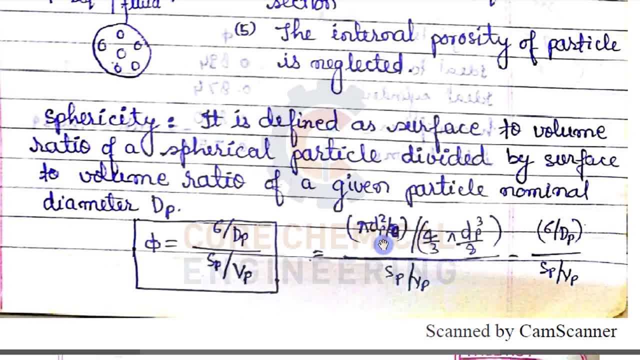 ok. divided by 4 by 3, pi, dp, cube by 8, ok. now whole divided by surface area to volume ratio, sp by bp. ok. now if you divide this value, ok, you will get 6 by dp. divided by sp by bp. ok, so this is your correct answer for calculation of sphericity, ok, 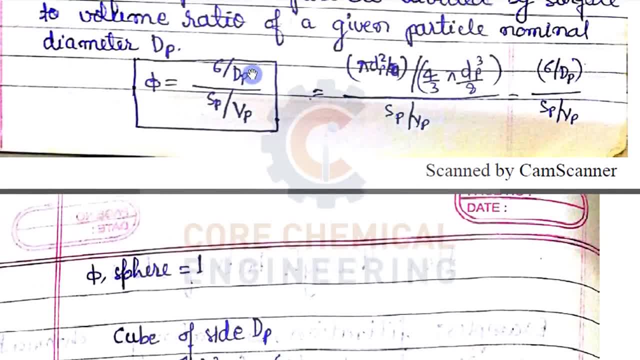 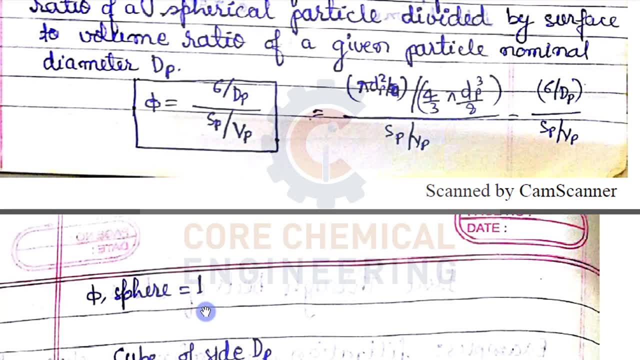 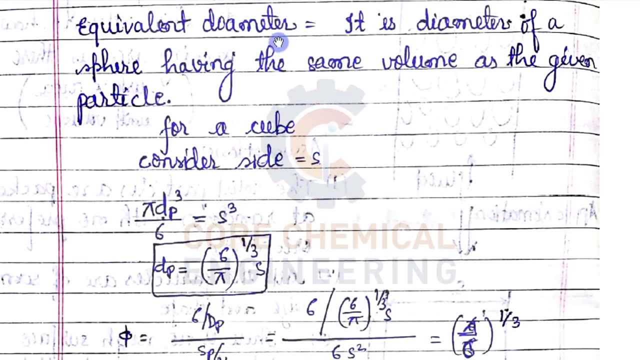 now, 5 is equal to 1. ok, so both will be same. if you are going to calculate the for sphere you are going to, you are comparing with the sphere only, so obviously it will be same. now, the next thing that we need to know is equivalent diameter, because these are the terms that we 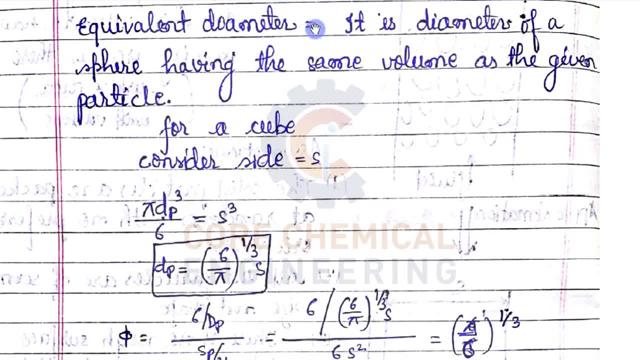 are going to use while the calculation of pressure drop. so equivalent diameter: it is diameter of a sphere having the same volume as a as the given particle. ok, so for a cube, consider side is having s, that cube is having side s, ok, so volume of the sphere has been. 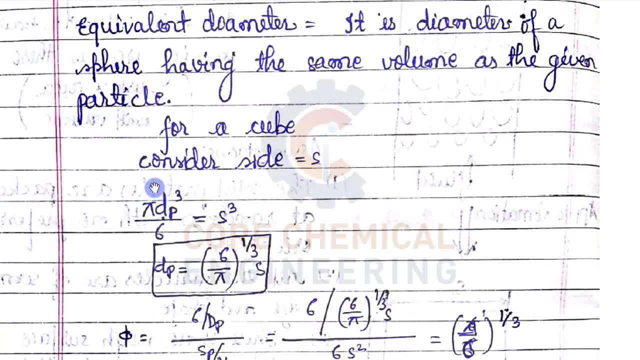 know, 4 upon 3, pi r cube is equivalent to pi d cube by 6, ok, is equal to s cube. now we will get dp in terms of side- ok, side of square, 6 by pi. lets do the power 1 by 3 into s now. 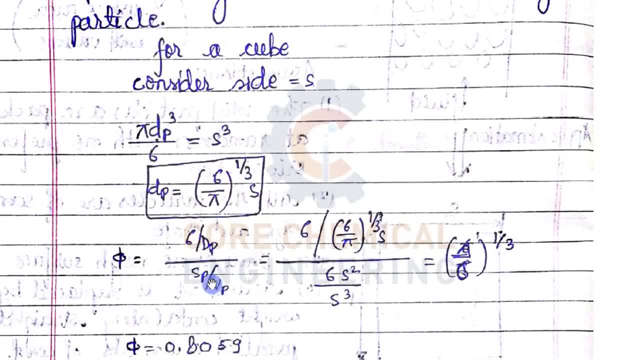 we have to calculate the sphericity now. 5 is equal to 6 by dp divided by sp, by avp. so 6 divided by dp, dp value. we have to use that. have calculated in the terms of side. ok, so let's put this value now. sp is your 6s square. 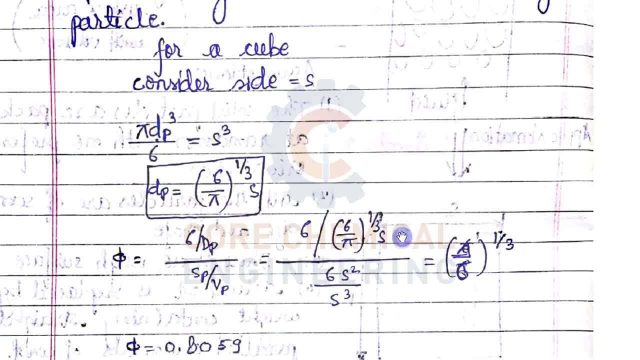 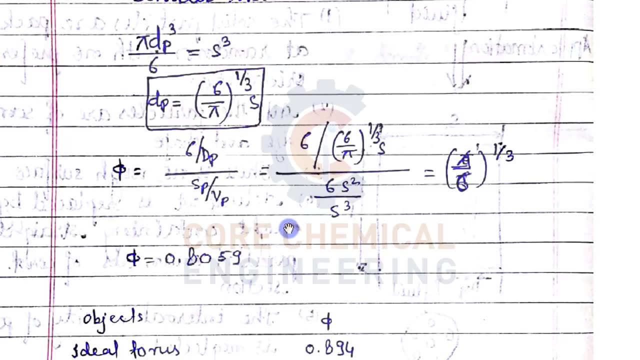 divided by volume, vp is your s cube. just if you solve this whole whole thing, ok term you will get pi by 6 raised to power 1, pi 3. now the value of pi is 0.8059. this is for cube. sometimes they give in the gate exam. they ask just simply: what is the sphericity of? 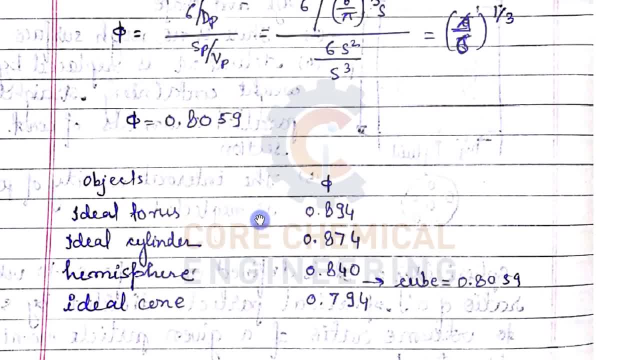 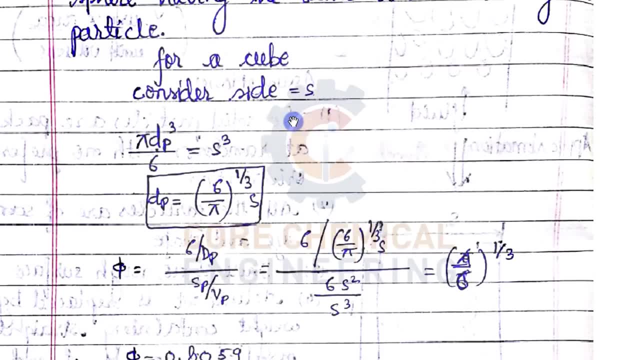 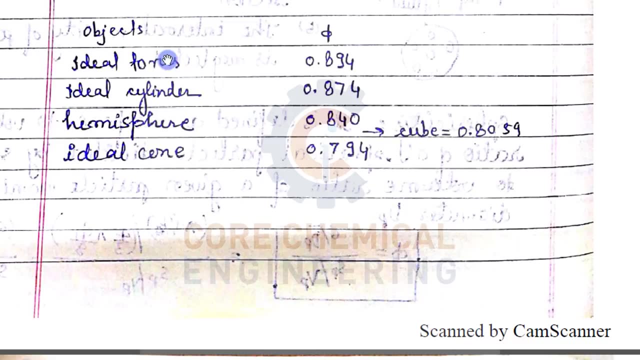 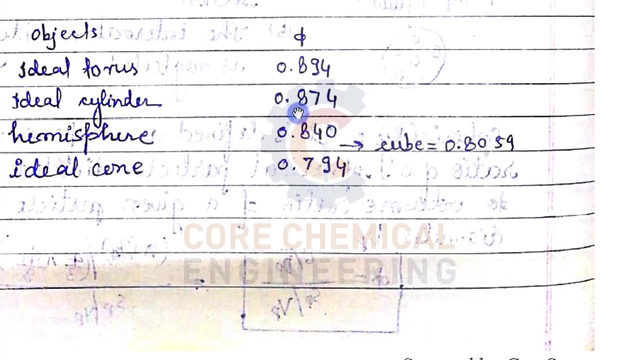 cube, ok. having having side s ok, or having side 5 cm unit, ok, so that dimension doesn't matter. your sphericity will be same, ok? pi is equal to 0.8059 now. the sphericity of other objects like radial torus is 0.896. radial cylinder is 0.874. hemisphere is 0.840 now. 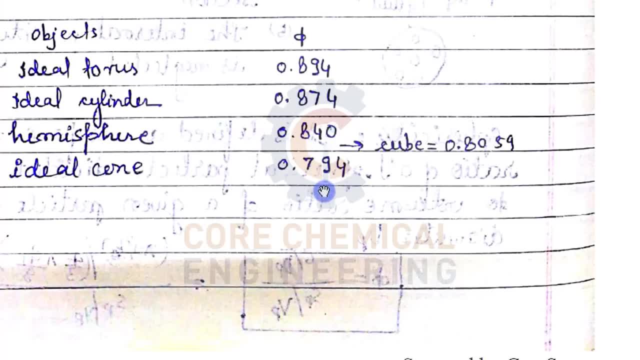 after that comes 0.8059, after that ideal cone 0.794. so you must remember the order. okay, order of increasing specificity or decreasing specificity with respect to the gate exam, because sometimes they give all this and they just ask the order of specificity in the gate exam. so if you are going to calculate, 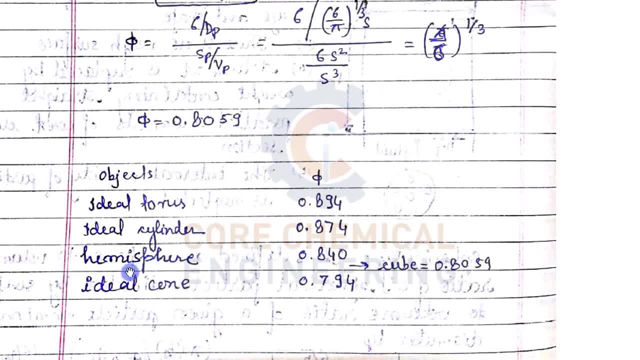 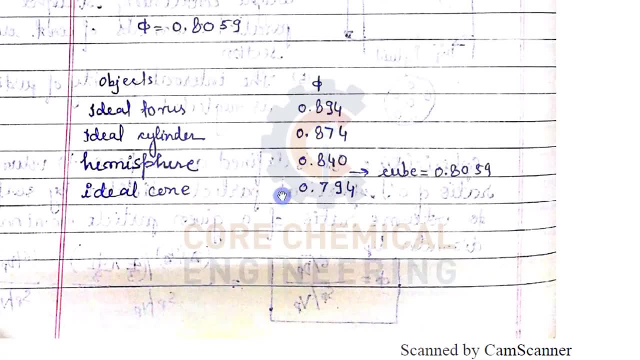 for each and everything like ideal cylinder, a hemisphere, then it is going to take it, take your time. so, in order to avoid the best days of time, you must remember this, at least for uh cylinder, hemisphere and cuban, cuban ideal can, ideal cone, you must remember. 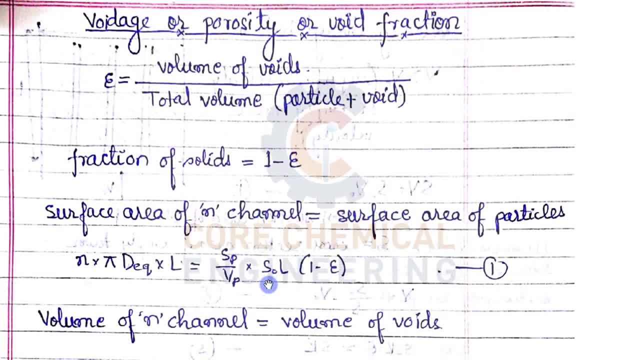 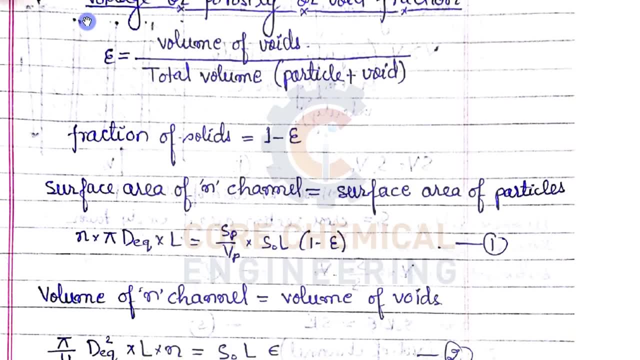 now let's go for the pressure drop- uh, pressure drop calculation part. okay, so you can see it here. y days are positive or white fraction, so we have to calculate first. so epsilon zero y days is equal to volume of wires divided by total volume volume. total volume is particle volume plus wide. okay, 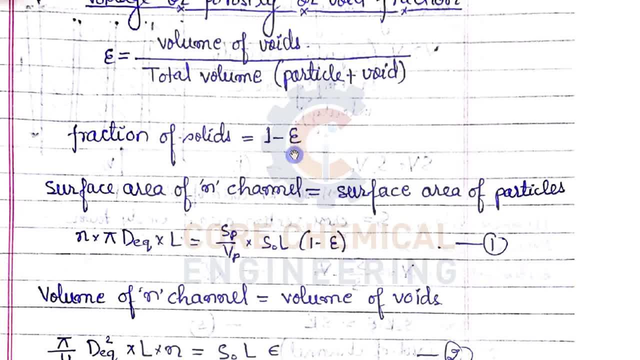 so fraction of solid is your, one minus epsilon wide is your. you will get the fraction of solid side. now, surface area of n channel is equal to surface area of particle, obviously. so, as we know, the surface area of n channel is equal to pi d equivalent. into l right, 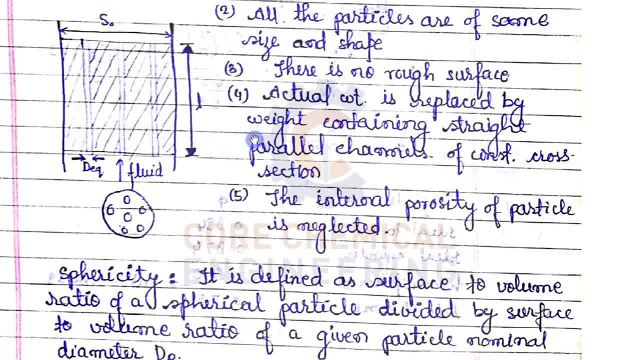 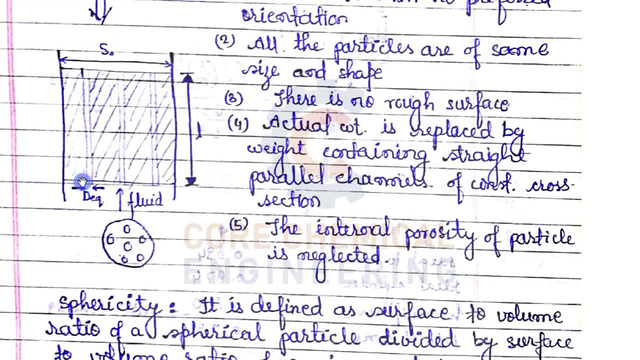 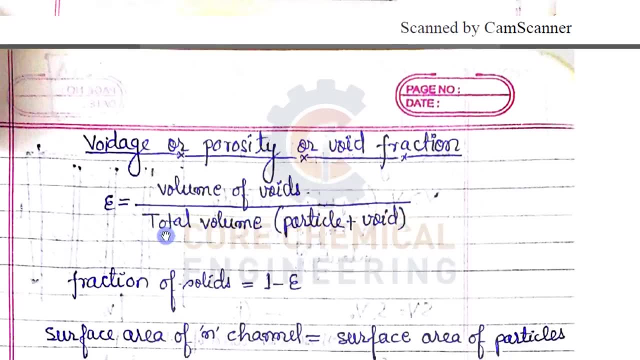 you will get pi d equivalent into l. this is your d equivalent diameter through which fluid is going to flow. okay, equivalent diameter. pi d equivalent equivalent into l, and l is the length of the bed. okay, so this is for one, one channel. if you multiply it with, 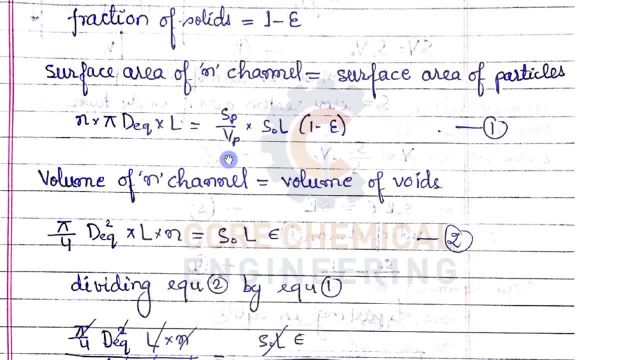 and you will get the surface area and channel now is equal to spy vp into, while this is the volume of solid epsilon. epsilon is, for Now, one minus epsilon is fraction of solid. okay, so you will find it here for one, one channel, and you will get the surface area of n channel now is equal to sppbp into. 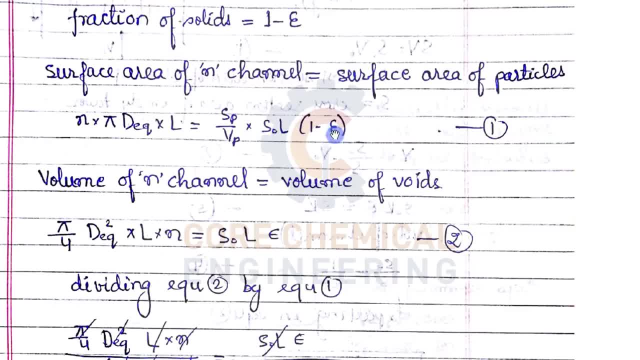 well, this is the volume of solid epsilon. epsilon is for wide, now one minus epsilon is fraction of solid. okay, so s not into. l is the total volume of solid, okay, so this is the equation. one now see the relation. volume of n channel is equal to volume of voids, as we know. so again, 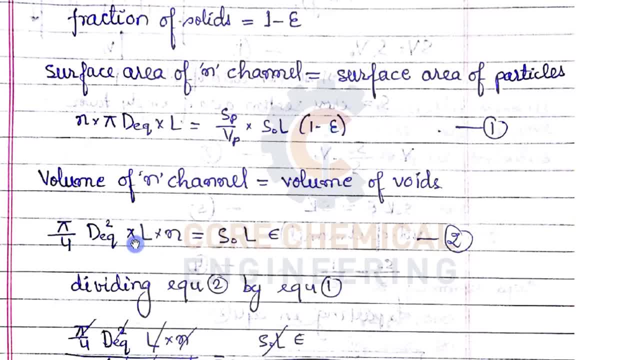 here by r square h. as we know, the the volume of any cylinder, okay, cylindrical, cylindrical form, okay now. so pi by four, d equivalent square into l is your volume of one channel. into n is correspond to volume of n channel, so is equal to s, not l. into epsilon: epsilon is. 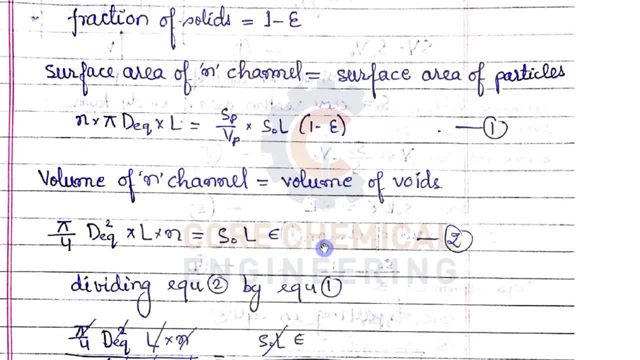 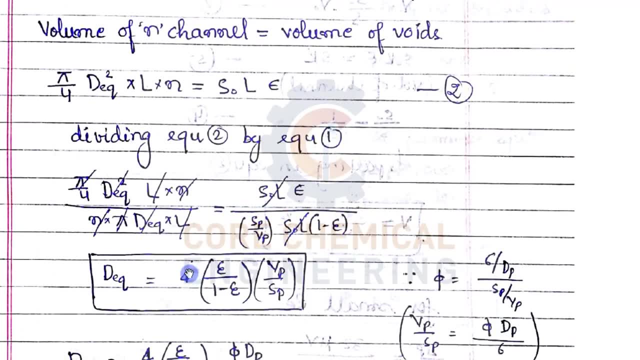 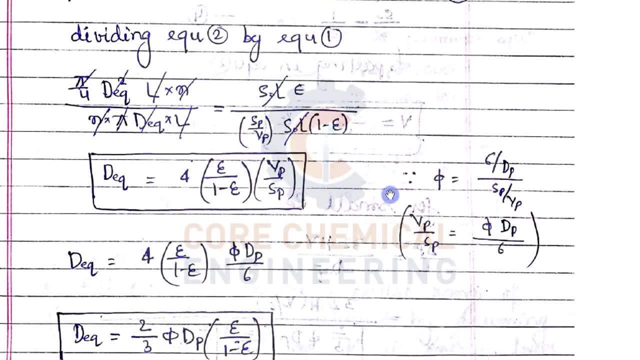 your wide, okay. so if you divide equation one by equation two by equation one, dividing equation two by equation one, and if you solve it, we will get the equivalent value is equal to four into epsilon divided by one minus epsilon, and break it into vp by sp. okay. so, as we know, 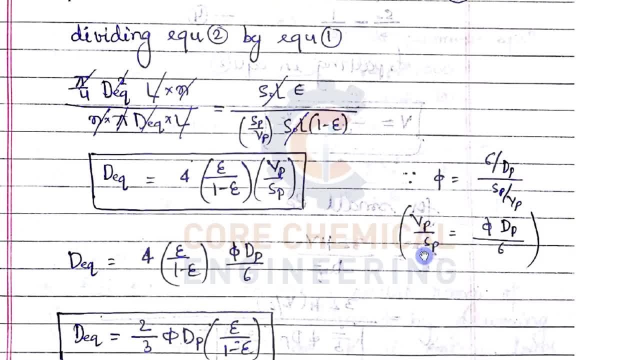 phi is equal to six by dp divided by sp by vp, so bp by sp. from here we can get phi, dp divided by six. So let's put this value here. so if you put this value- vp by sp from here to here, we will get the value of d. equivalent is equal to four into epsilon divided by one minus epsilon. 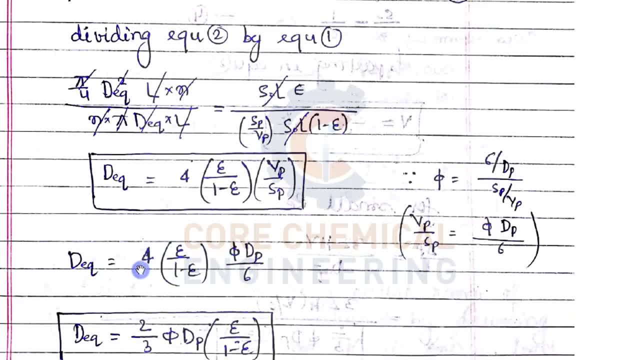 into phi dp divided by six. so if you solve it to divide both by two, two okay, so two here. three comes here. so d equivalent equal to two by three into phi dp, into epsilon divided by one minus epsilon. so this is the equivalent diameter. okay, for the channel calculation. 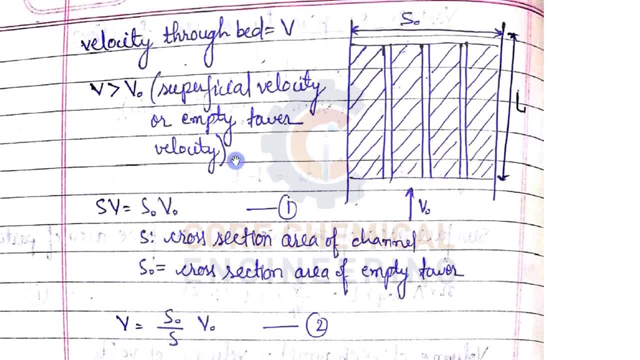 of equivalent diameter. Now comes the velocity through. width is equal to v. okay, so v will equal to v, not. okay, so v not is the initial approach. velocity, now the velocity that will flow into the channel. so area here gets decrease, okay, so anyway, pressure will. area gets decrease, then your. 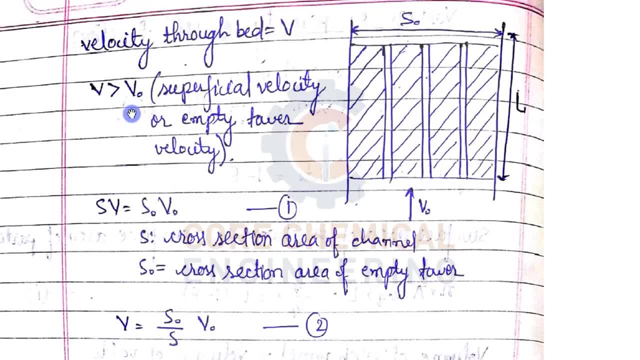 velocity will increase, right, so v is equal to greater than v. not so superficial velocity are impacted, our velocity v not. So as we know, according to continuity equation, a one v one area into velocity at one point is equal to a two into v. two, okay, right area at other point into velocity. so similarly. 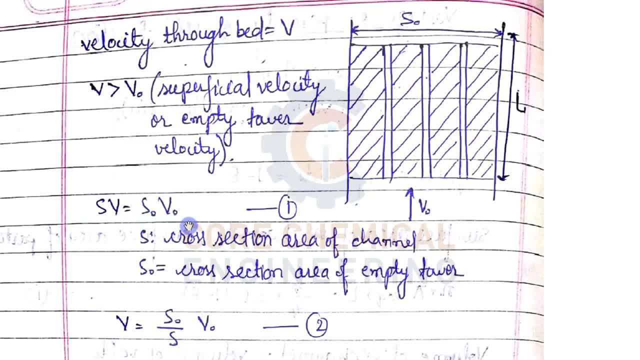 that is, here is the relation: s into v is equal to s, not into v not. s is cross section area of channel, s not is cross section area of empty tower. so if you are taking cross section of area of empty tower then v not is the velocity here. if you are taking cross section area, 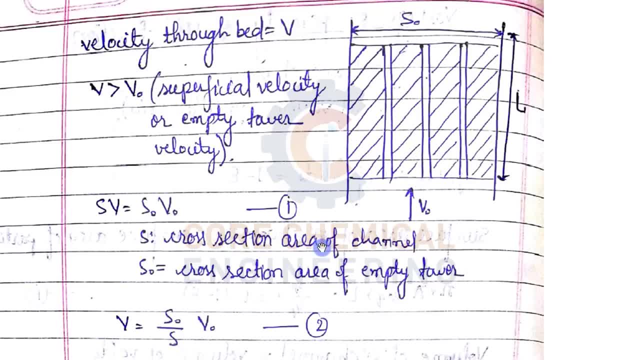 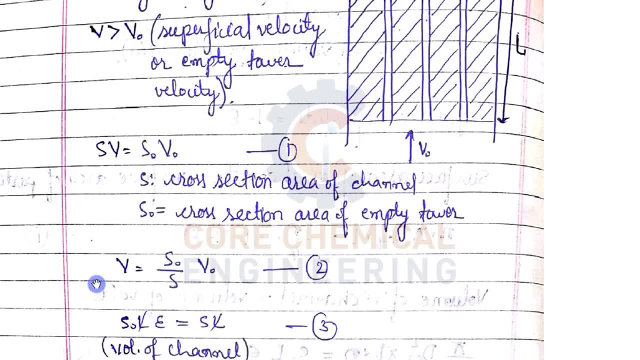 s here, only Cross section, cross section, cross section, area of channel. okay, if you are taking edges, then we need to consider volume with respect to the s. okay, velocity with respect to s. so v is equal to s, not divided by s into v, not so, as we know, volume of channel: okay, so volume, 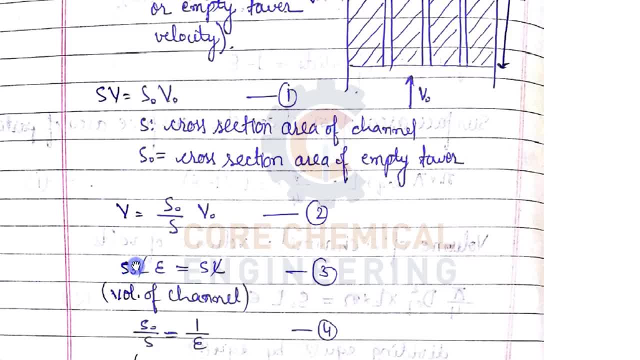 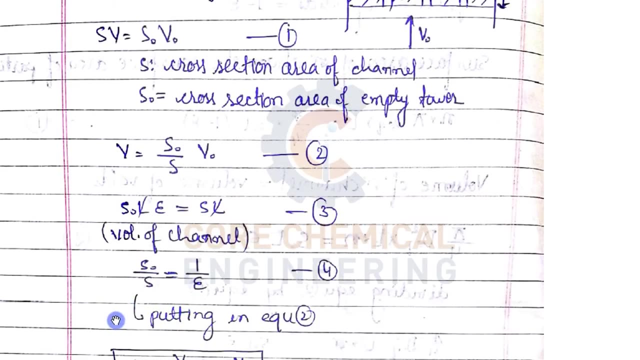 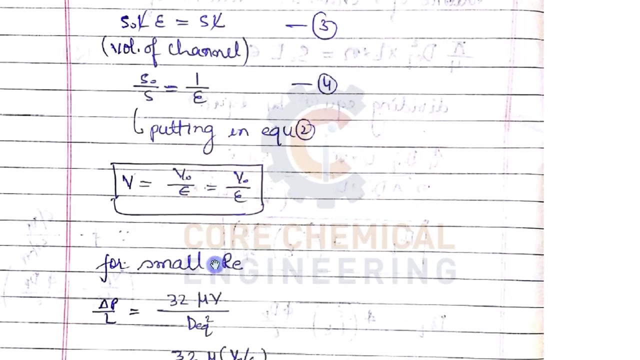 of channel s into l is equal to s into l into epsilon. epsilon is your empty part, so it becomes the volume of the channel. So S not divided by s equal to one by epsilon. so if you put the value of s here, you will get v equal to v not divided by epsilon is equal to same v, not by epsilon. okay, so for 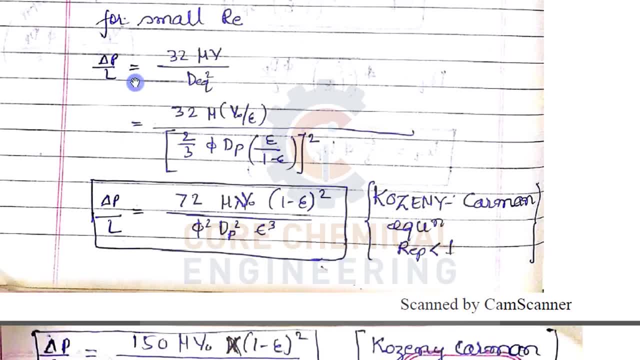 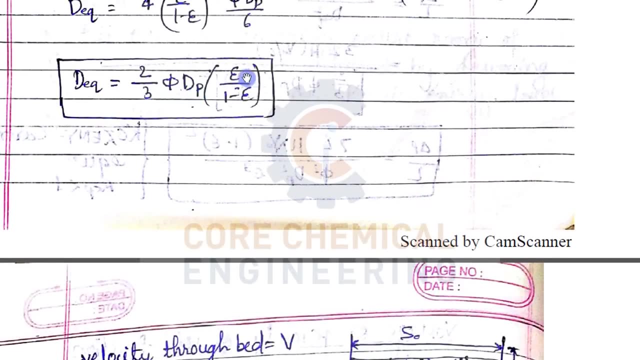 small Reynolds number. as we know, delta p by l is equal to thirty two mu v divided by d covalent square. okay, so d covalent value, we had calculated it here. okay, d covalent by s equal to two by three, into five, into dp, into epsilon, dot by one minus epsilon. now, 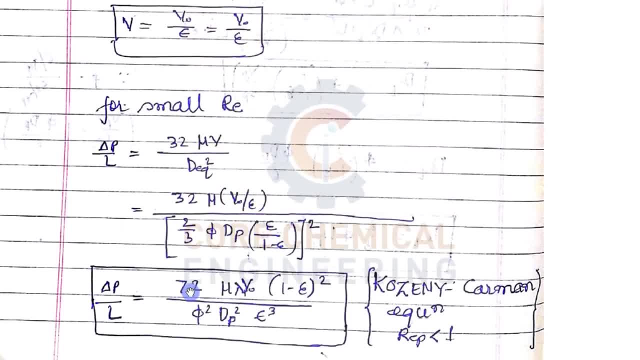 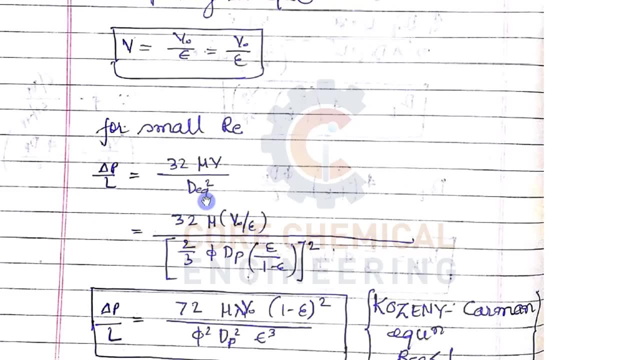 you have to put this d covalent value in this question here, okay, in the hazard, hazard posley equation, when your Reynolds number is less than one, okay, then only this relation is varied, so put the value of d covalent here. if you put the value of d covalent here, four square. 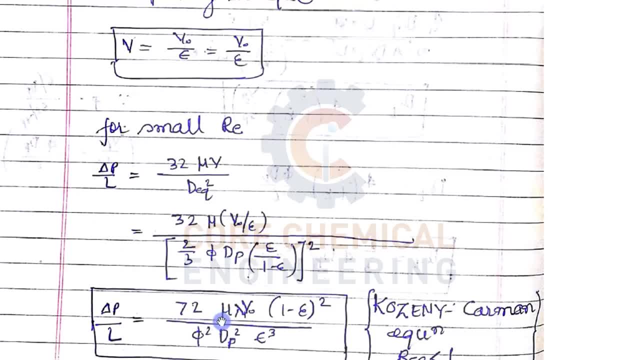 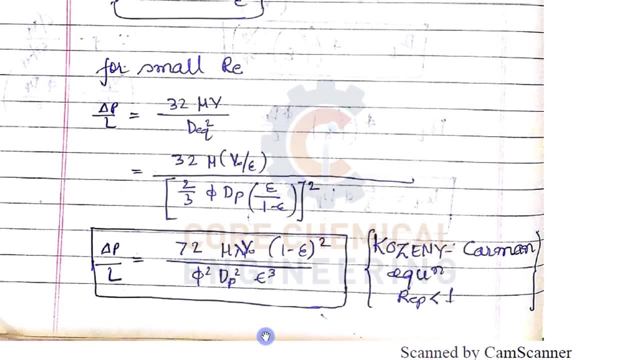 you will get the final value. this delta p by l is equal to seventy two mu lambda. one p square into epsilon cube. so this is called kozeny carmen equation. when we lost kozeny carmen equation, and this equation is valid when reynolds number is less than one, because 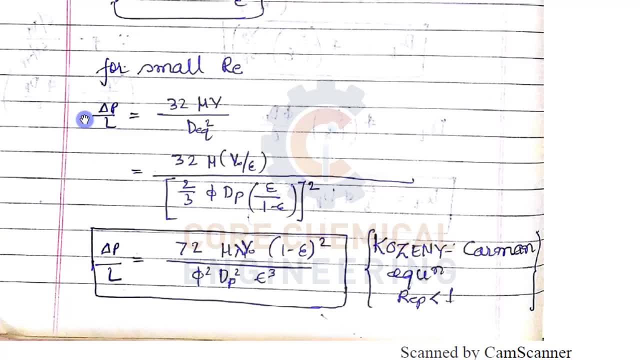 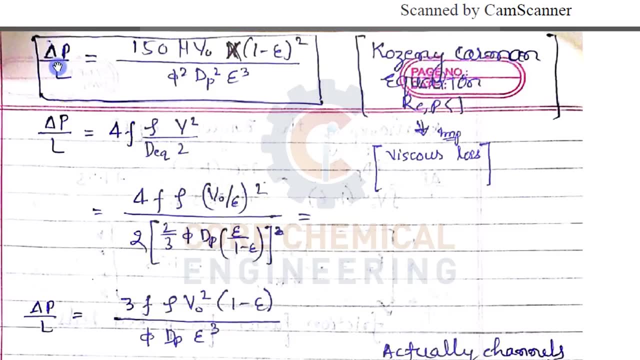 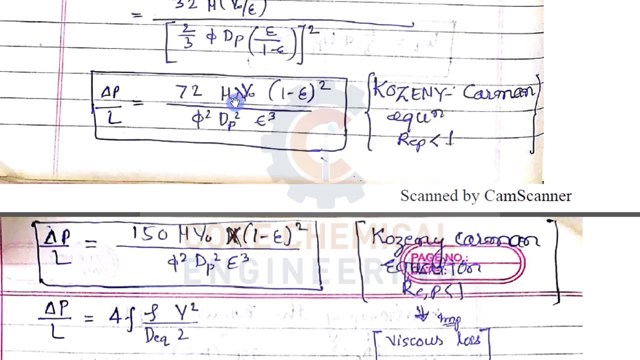 for the small, for a small, uh, reynolds number only. this relation hasn't posed the equation is valid. okay now, so this is your relation. delta p by l is equal to one fifty now, so lambda one, the value we have taken from the experiment. we got that, this value, okay, lambda. 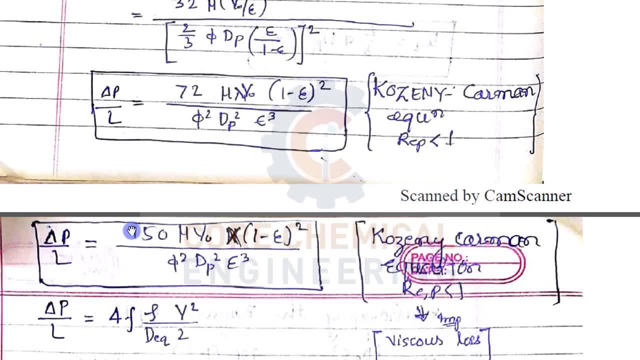 one into seventy two is equal to into seventy two. value is equal to your one fifty. okay, so delta p by l is equal to one fifty. mu v naught into one minus epsilon square divided by phi square, dp square into epsilon cube. so this is the formula relation for kozeny. 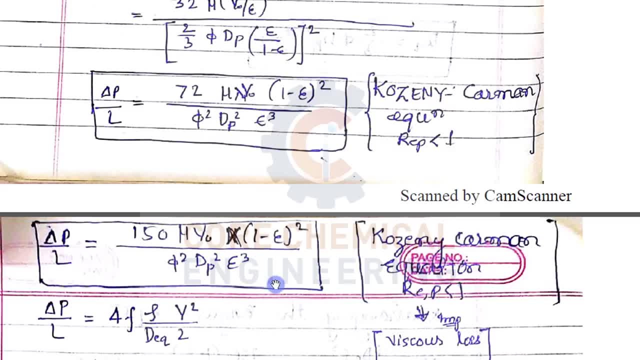 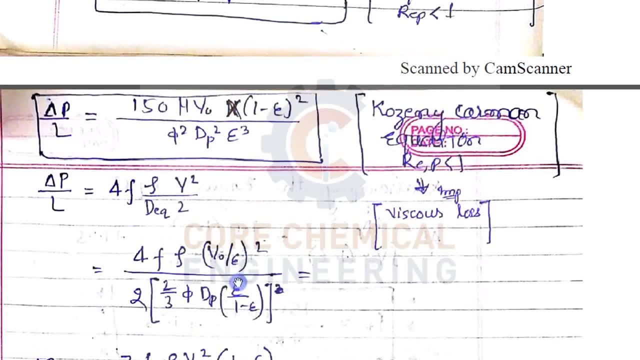 carmen equation for reynolds, number less than one. okay, so this one is very, very important, you must remember. sometimes they ask the question in the gate exam directly based on this formula. okay, now, as we know, the for turbulent case. okay, delta p by l is equal to one into seventy two. okay, so delta p by l is equal to one fifty. 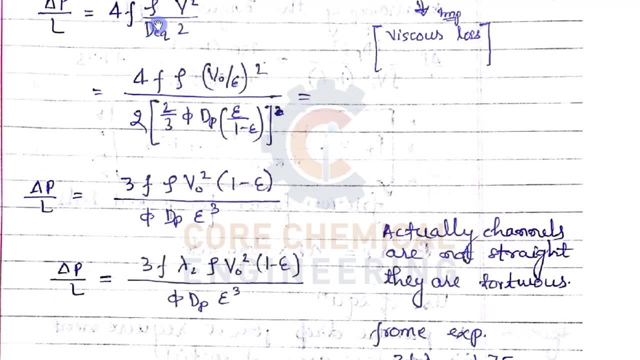 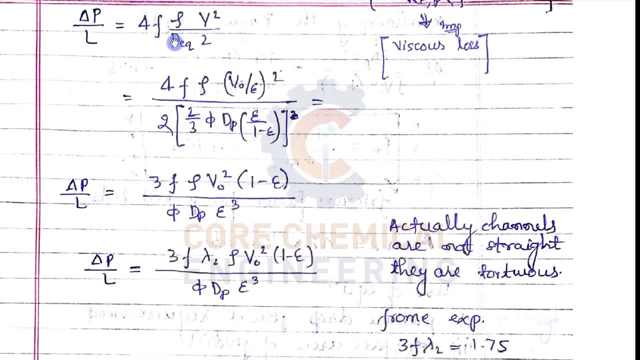 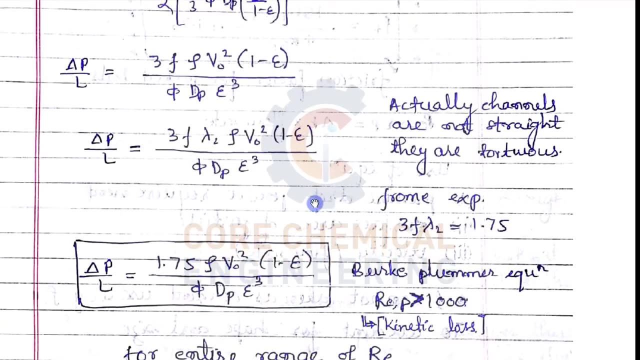 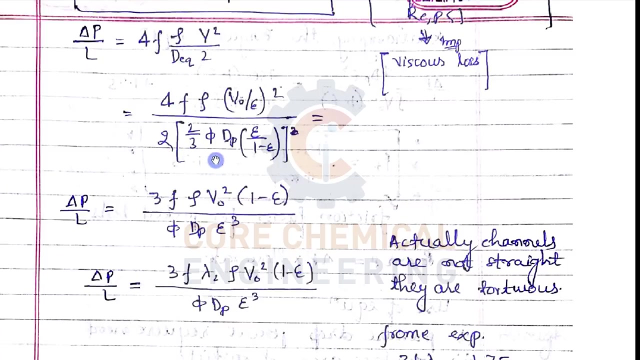 one is equal to four f. okay, four f, uh. rho v square by two. d equivalent delta p by l is equal to four f. rho v square by two into d equivalent here. okay, now, d equivalent value again. we need to put it here: if you put now, now, if you put the value of d equivalent, okay, uh, d equivalent value two by three pi. 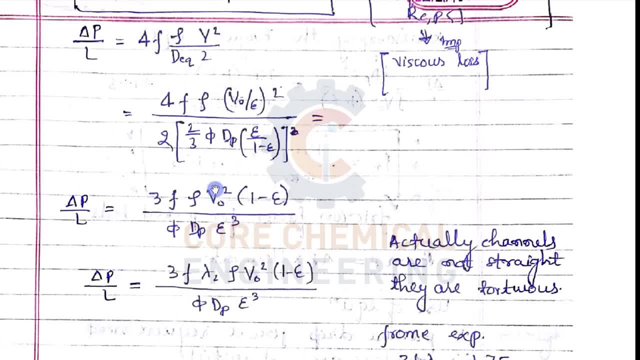 into dp into epsilon divided by one minus two, into dp, into epsilon divided by one minus epsilon. if you solve it, you will get the this value okay. delta p by l is equal to three. f rho v naught square into one minus epsilon divided by five dp into epsilon cube, okay. 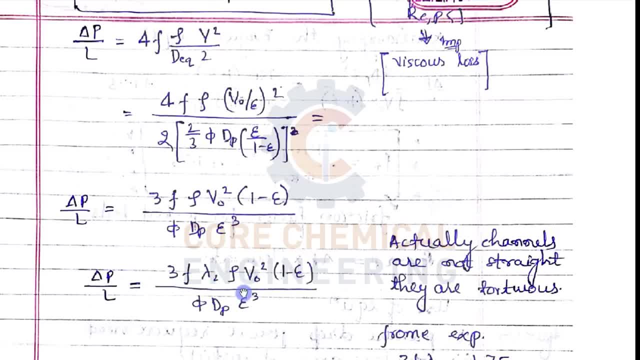 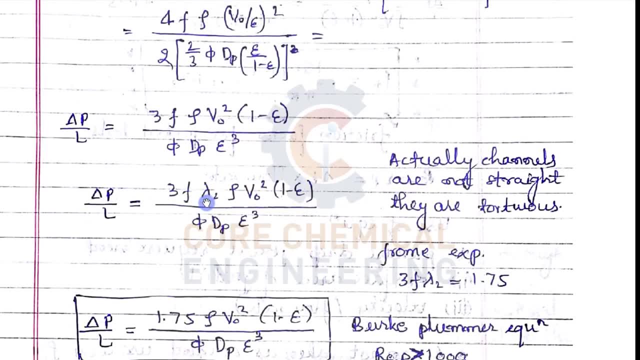 so delta p by l is equal to three f lambda two into rho v naught square, into one minus epsilon divided by five dp epsilon cube. so three f lambda two, okay, okay, lambda two. we are taking as constant constant like uh one, constant that uh equal. that actually makes. 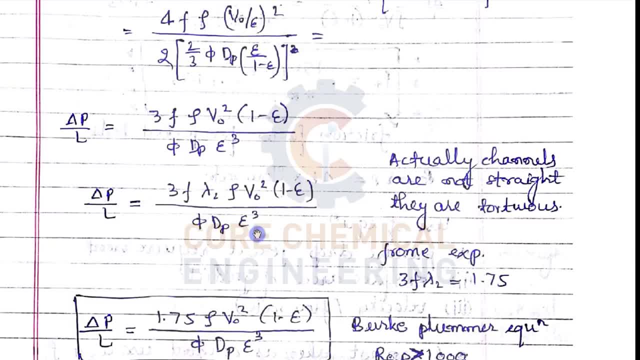 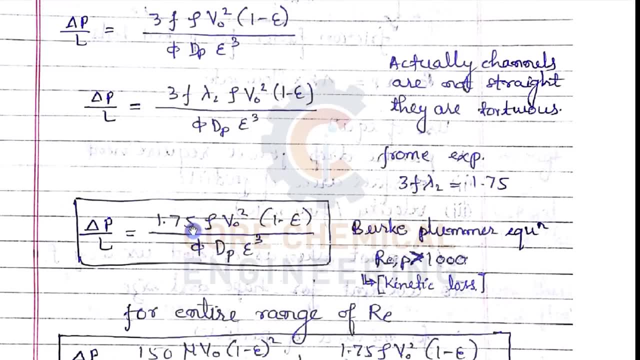 it choice where left hand and right hand, uh, equal. okay, so three f lambda 2 value. from the experiment we have gotten one point seven five. so if you put this value we'll get delta p by l is equal to one point seven five into rho v naught square into one minus epsilon. 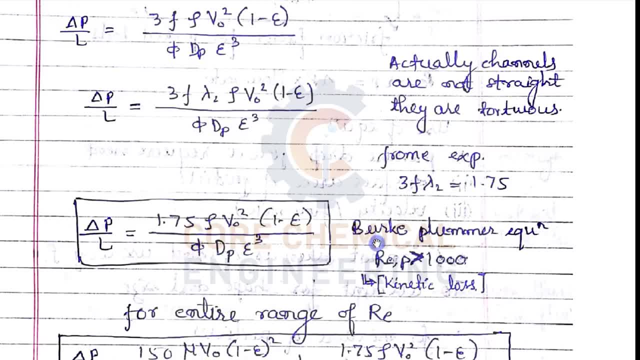 divided by 5dp into free q. so this relation is called as bulk plumber equation, and that is valid for ren는데요 greater than thousand. okay, so this is called kinetic loss. okay, and this one is called viscous loss. okay, to make a plasma star, or Nash's fraternity, if you all. 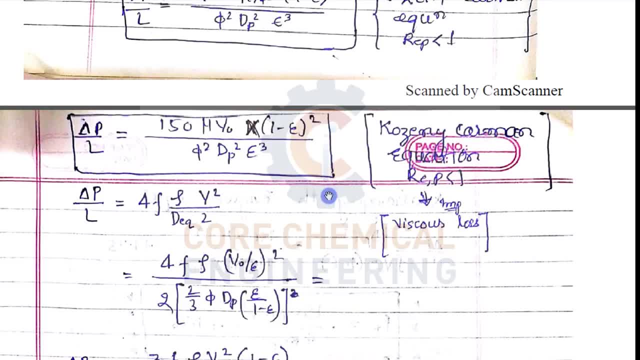 read the numbers you should see that you couldn't big up the so theicking. this was before. it was the government who has the same, slowly it had a little more problem is wanting to move across here. loss: sometimes in the gate exam they are asked which term is viscous loss and which term. 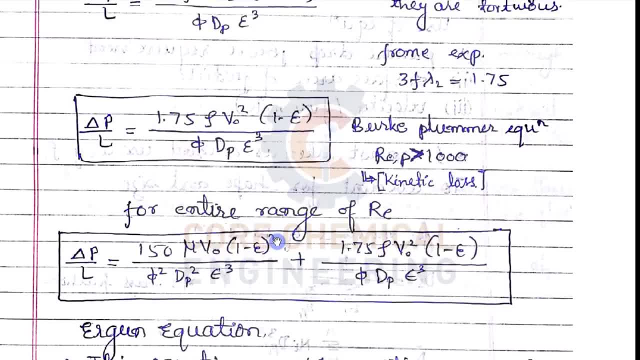 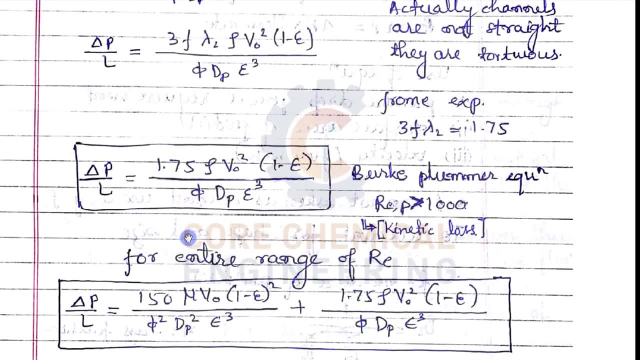 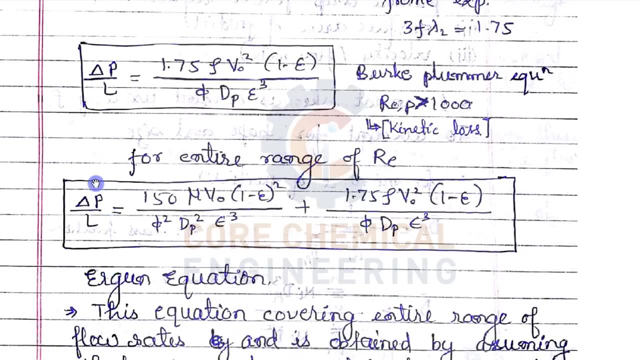 is kinetic loss, you must remember. ok, now, for entire range of reynolds number you have to add both the kinetic and viscous loss, ok, so if you add it you will get this whole term. ok, so this equation is called as argon equation. so delta p by l is equal to one fifty mu b. 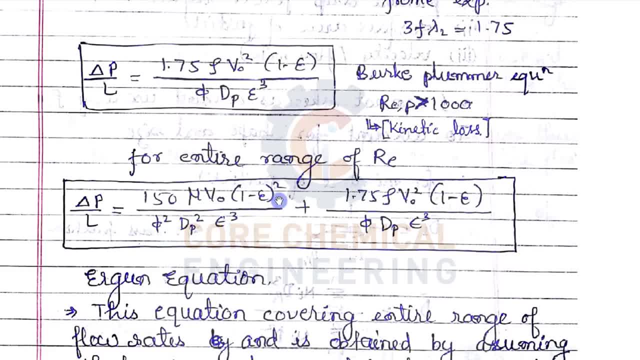 naught into one minus epsilon square divided by five square dp square, epsilon cube. this is your viscous loss, plus one point seven, five rho v naught square into one minus epsilon divided by five dp, into epsilon cube. ok, this is your kinetic loss. ok, so if you add both, 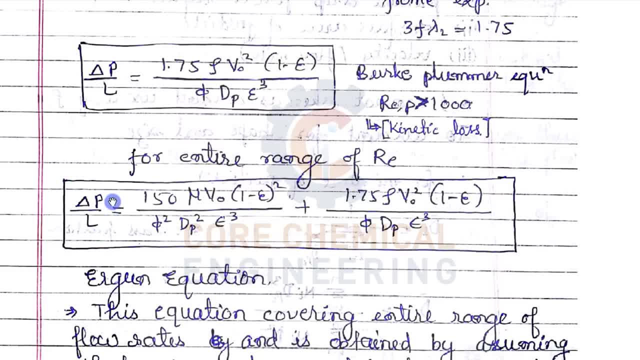 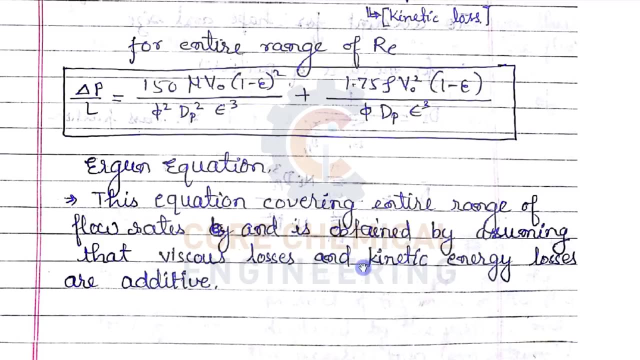 the term you will get the pressure drop through the pint bed of length l, ok. height l for the entire range of reynolds, number, ok, so this is very important. so this equation covering entire range of flow rates and is obtained by assuming the viscous loss and kinetic energy losses are additive, ok. 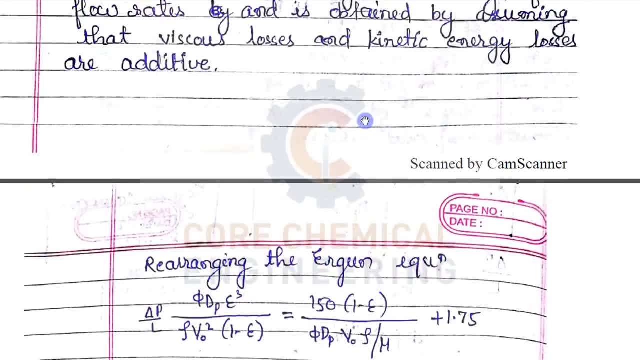 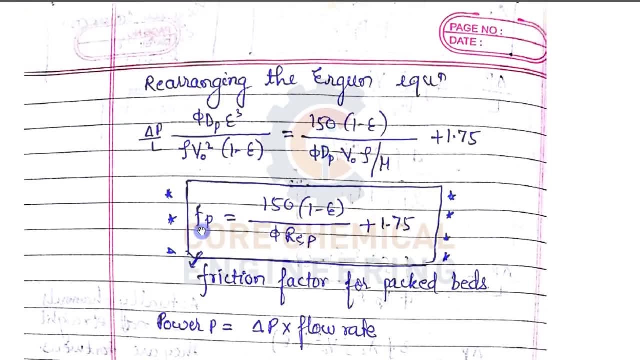 so rearranging the equation: ok, one point seven, five, keep the term here ok, and divide the whole term by this value, we will get this relation ok. so from here we will get f? v equal to one fifty into one minus epsilon divided by five into reynolds, number of particle plus. 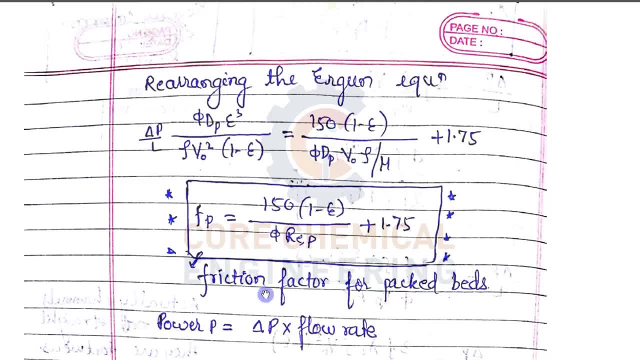 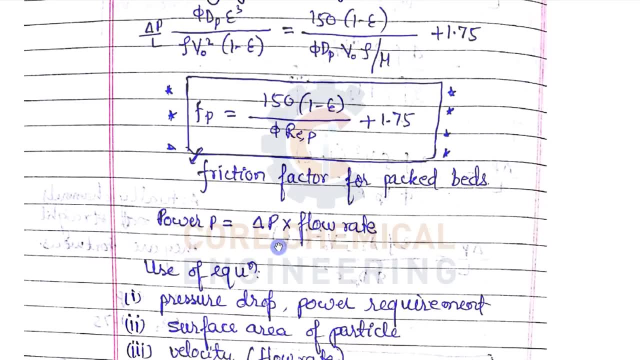 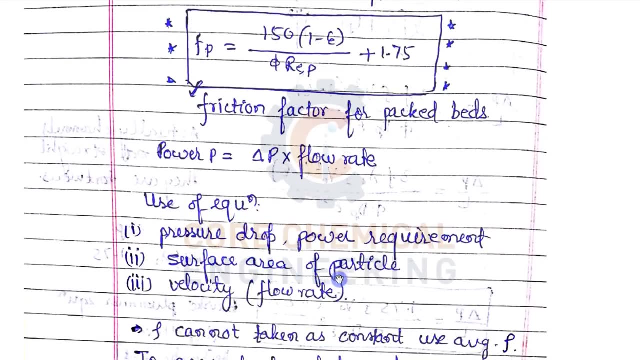 one point seven, five. ok, so friction factor, for this is called friction factor for the packed bed, right, so there were. from there we can calculate the power is equal to delta p into flow rate. ok, so use of this equation is to calculate pressure drop. power requirement. surface area: 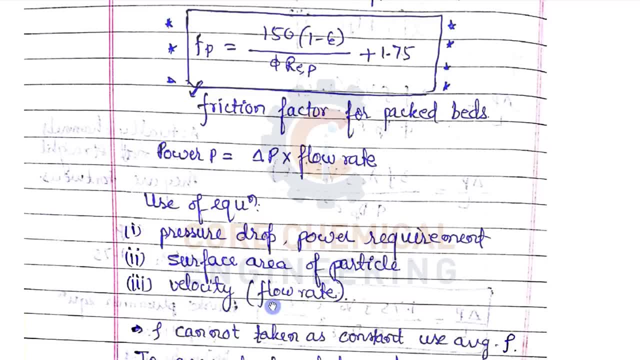 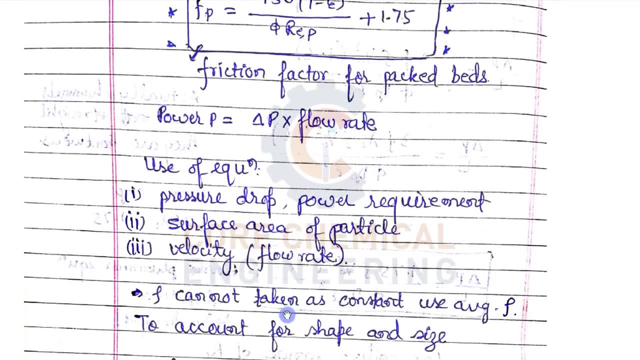 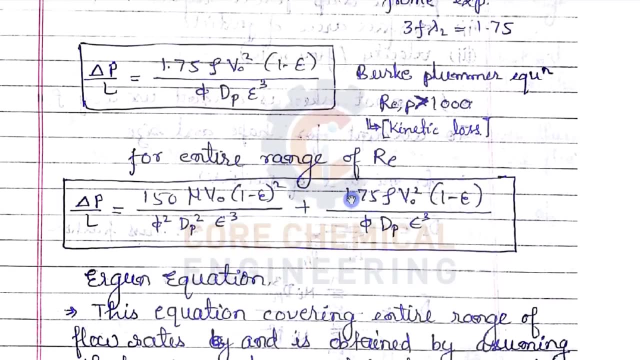 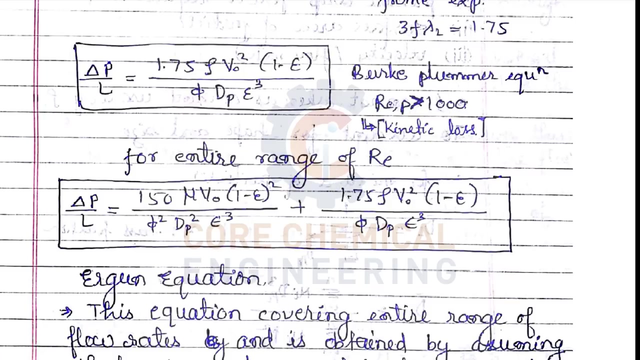 of particle velocity for calculation of flow rate. ok, so rho cannot be taken as constant. use average rho to account. account for the shape and size of particle. ok, so, guys, this is all about the calculation of pressure drop through the packed beds. ok, so, guys, this is all about the pressure drop calculation across the packed beds. ok, so you must remember this.